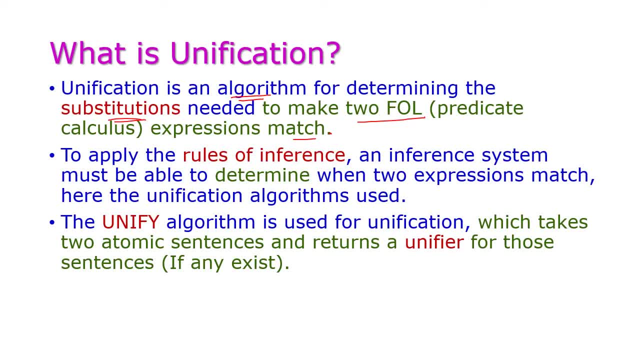 That is, we are going to match two first order logic expressions, alpha and beta, by using this substitution theta To apply the inference rules. the inference system must be able to determine when two expressions will match, So in that situation we can use this unification algorithms. 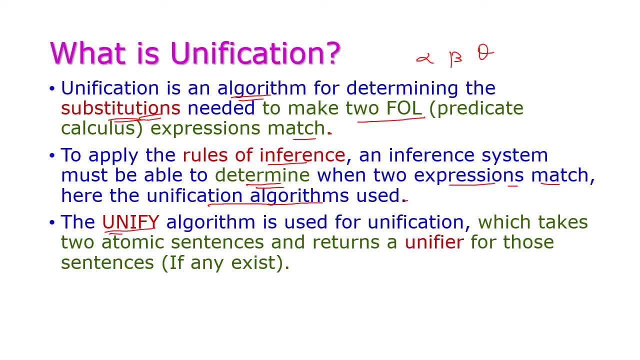 Here the algorithm unify, which is used for unification, Which determines the first order logic expression. This takes two atomic sentences, alpha and beta, and return the unifier theta for those sentences. if any exist, That is, if these systems match each other, then this will return the unifier. Otherwise it will return failure message. 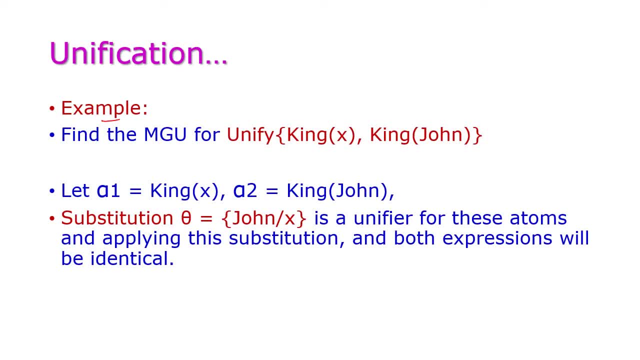 Let us see one example for this unification. Here find the most general unifier: mgU. mgU means most general unifier for these sentences. this is alpha and this is beta. Unifier of king x comma king john. Here alpha 1 is king of x and alpha 2 is king of john. 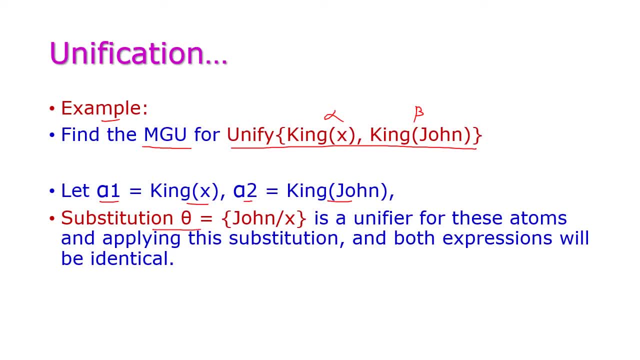 Next, we have to apply the substitution here: Theta, that is john gives x, That is, in the place of x, we have to substitute. Okay, then we make, these two sentences will be equal right. So substitution theta is equal to john gives. x is unifier for those atoms, that is, atomic statements, and applying this substitution and both expressions will be identical. 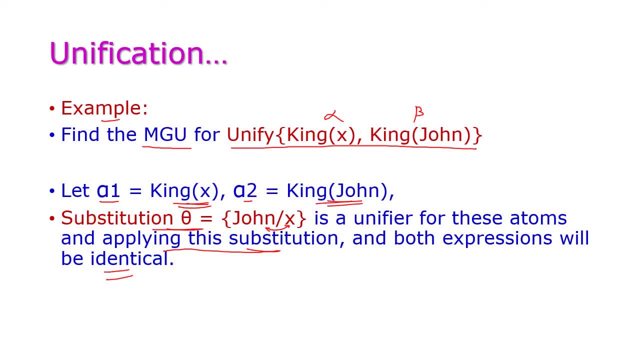 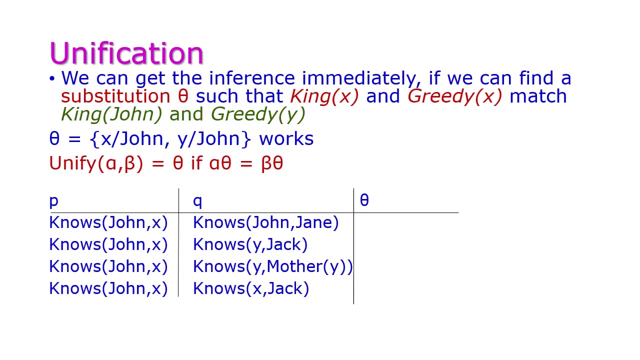 Okay, so after converting this x with john, Now king of john, which is equal to king of john. Okay, so alpha 1 is equal to alpha 2.. This is what substitution. By using unification, we can get inferences immediately. if we can find a substitution, theta right. 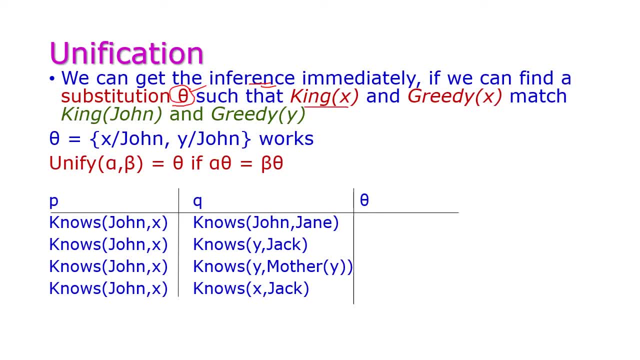 So such that king of X and greedy of x. Here we are having the variable x and x, which match king of john and greedy of y. Okay, so what is the substitution here? X that gives john and y gives john. then it will work. 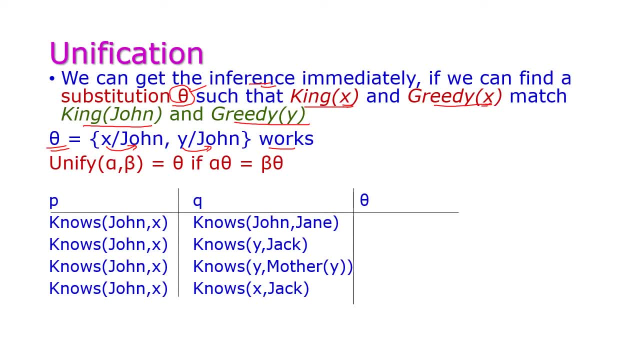 That is, when we make these two statements equal, then we have to map the variables with the corresponding values. Okay, King of X and greedy of x, which is equal to king of john, and greedy of y. Okay, then x is equal to john, as well as y is also equal to john, right, 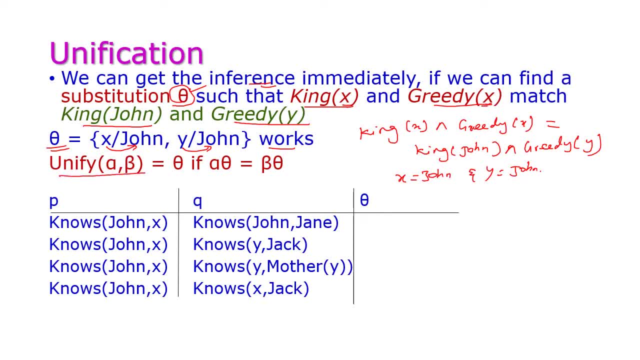 Okay, so here we are going to unify alpha and beta. okay, this is alpha and this is beta, with theta, if alpha theta which is equal to beta theta, that is, we are going to substitute the same value of these two statements. okay, first order logic statement. Let us see examples for this. the first one is nose of john, comma x. 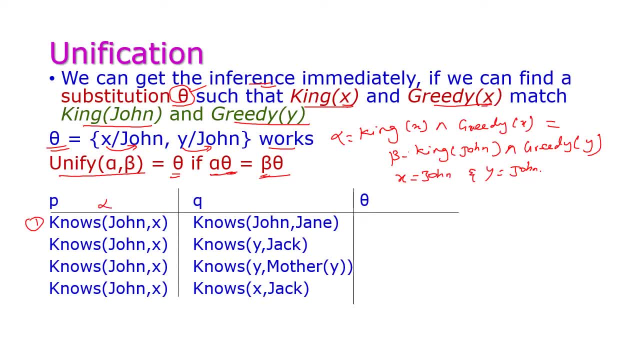 This is the first statement. For example, alpha and p. this is the another statement, that is, for example, beta. okay, These two are equal right. nose of john comma j, nose of john comma j. Then what is x? here we are having a variable x, isn't it? then what is x? when x is equal to x gives j. then these two, that is, p equal to q. 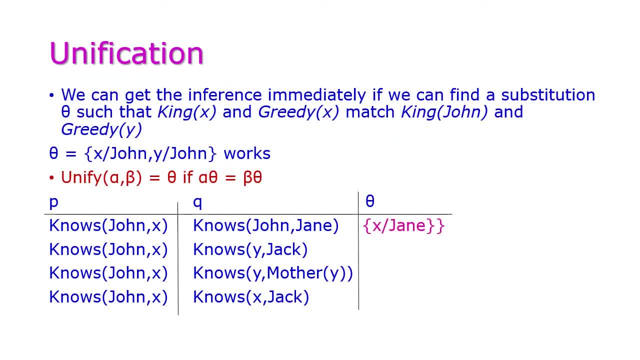 Okay, see, x is substituted with j. and when come to the next statement, nose of john comma x, and second one is nose of y comma jack. okay, now, here we are having two different variables, x and y, and two different values, also, john and jack. Now what is the x value and what is y value?